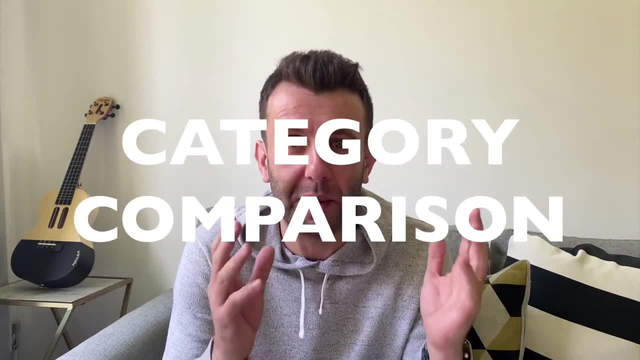 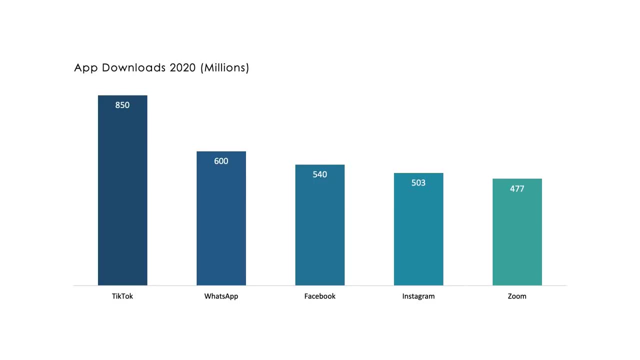 main types. Vertical bar charts are the best for category comparison. so if you're comparing countries or teams- and in this example we're looking at different apps and how many downloads there were in 2020.. With bar charts, we can quickly and easily compare the differences in. 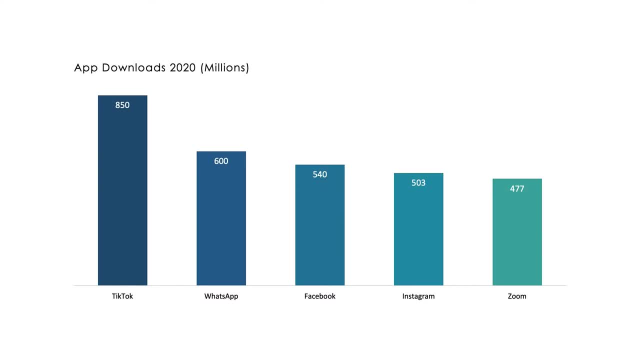 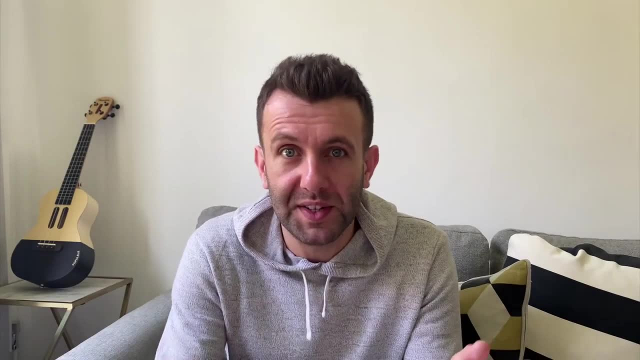 data, with the story in this one being that, despite what most people think, TikTok- not Zoom- was the most downloaded app of 2020.. But vertical bar charts lose that quick comparability when there's lots of different categories, so try and only use them if there's less than seven categories. 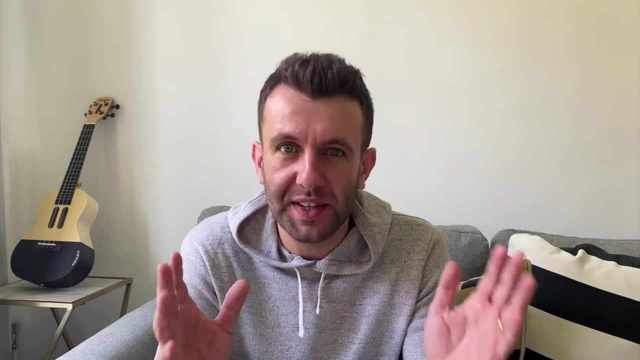 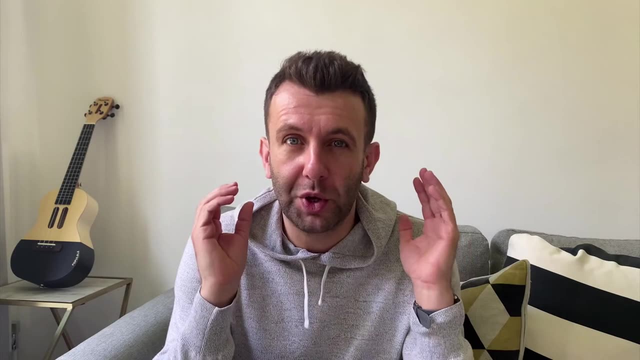 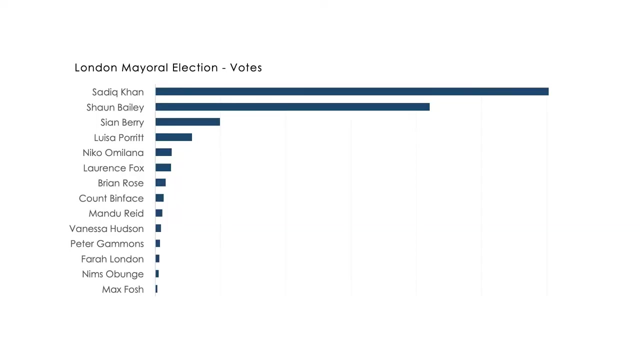 However, if you absolutely must have between seven and fifteen different data points, flip your vertical bar chart on its side and you have a horizontal bar chart. Really, though, the best when you want to communicate ranking. so things like election results, like this chart about the London mayoral elections that shows the candidates ranked by votes, They're also great for. 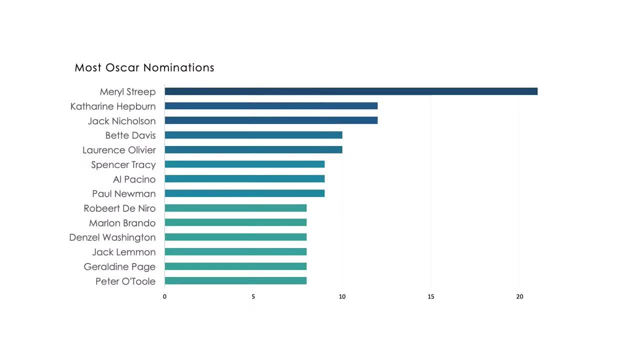 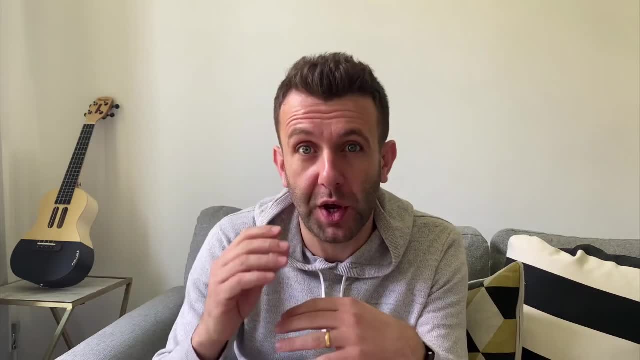 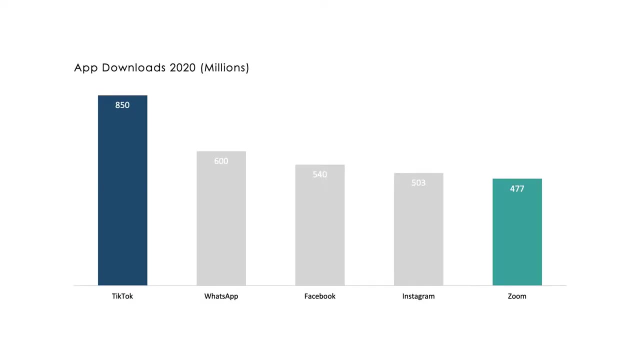 showing things like performance stats, like sales performance, or this example here which shows Oscar nomination performance. You should use stacked bar charts if you want to show part to whole. so how much different elements contribute to that overall total? For example, we already showed this chart where the main message was that TikTok, not Zoom, was the most downloaded app. 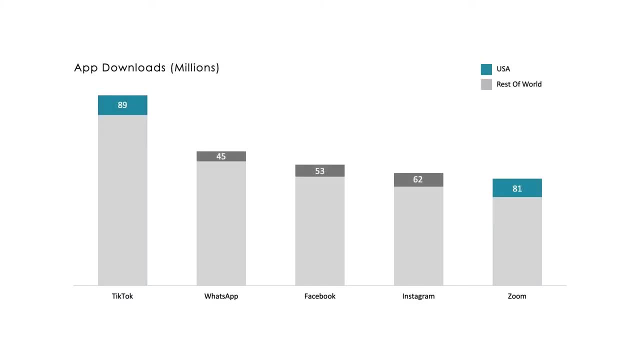 If you were then to use a stacked bar chart and break out the downloads for the US, you still get the overall picture, but you also see that in the US the difference between the two is actually a lot smaller, which is probably why people thought that zoom was more popular. 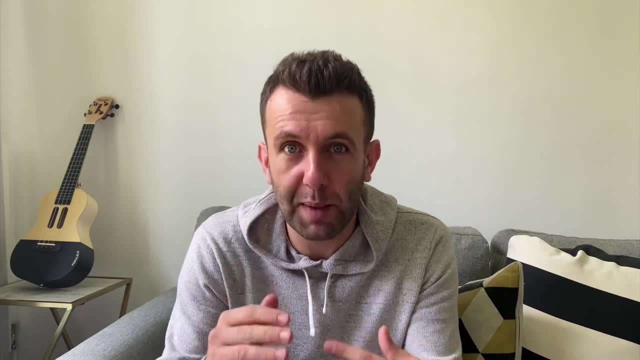 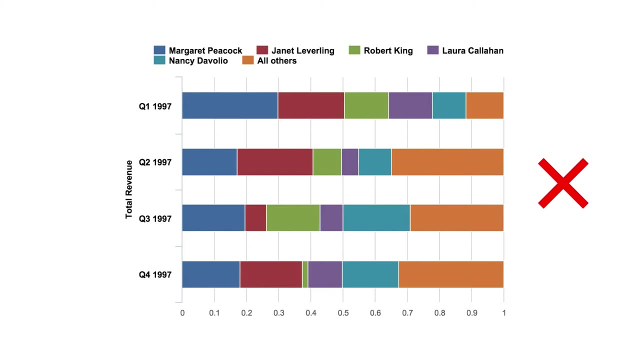 A warning though, for stacked bar charts, to keep them simple. as soon as the stacked bar chart becomes far too complicated, like this one, comparing the different components becomes almost impossible and they become more or less useless. So that's bar charts. Now for the second most popular chart in the world, which is the histogram. 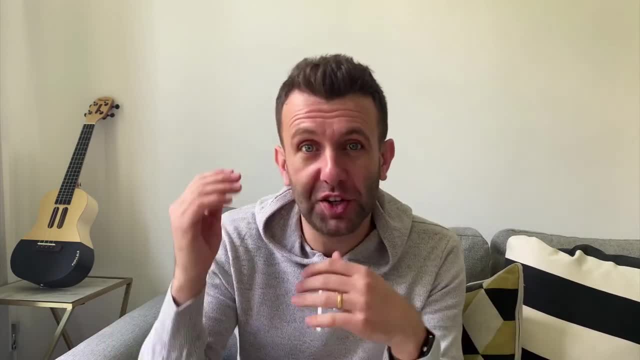 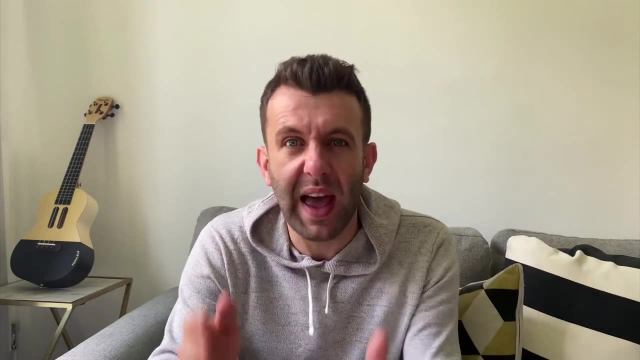 which is basically a bar chart. But if a bar chart breaks down data by different categories, histograms should show the distribution over a continuous variable. So things like time, age, weight. These charts are great to understand, things like this one showing the income distribution in the US. 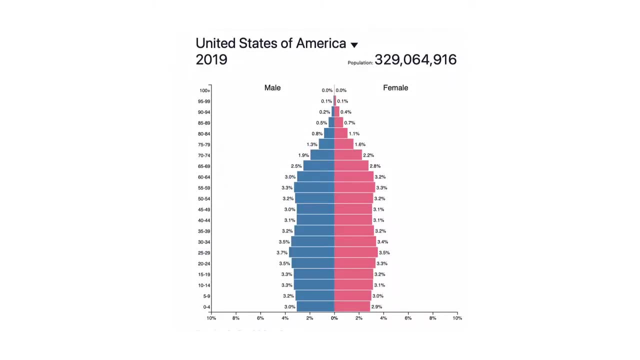 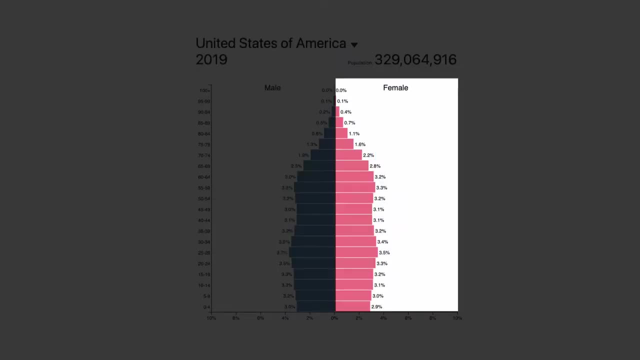 and probably most famously, population distribution Like this one showing data for the US, where age is on the y-axis and population on the x-axis. It's split by male and female, And histograms are generally less about the individual data points, more about the broader pattern that it shows. 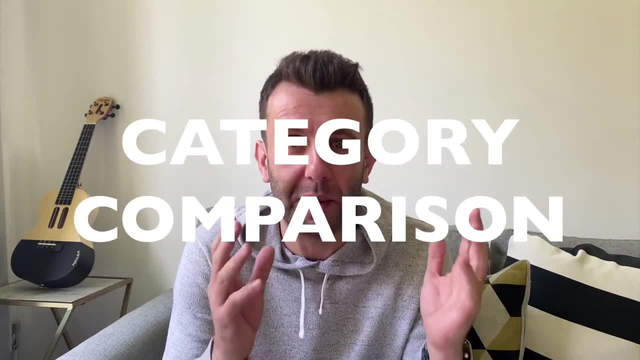 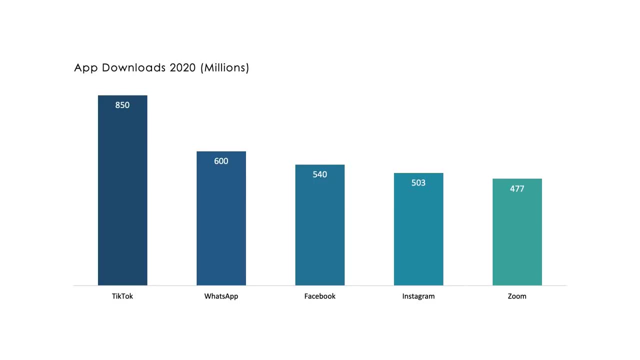 main types. Vertical bar charts are the best for category comparison. so if you're comparing countries or teams- and in this example we're looking at different apps and how many downloads there were in 2020.. With bar charts, we can quickly and easily compare the differences in. 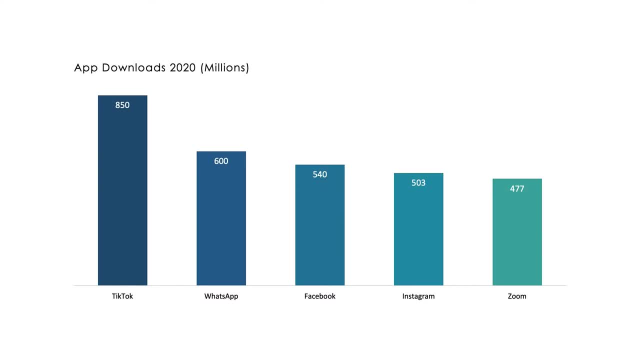 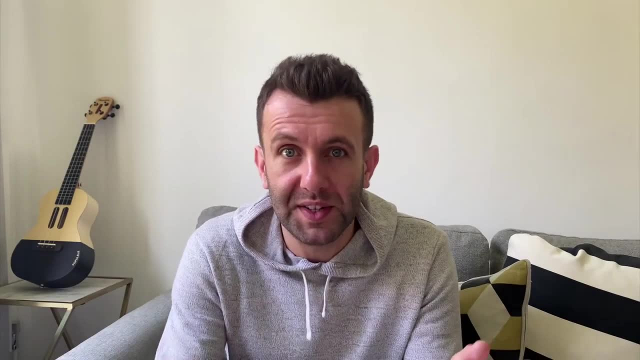 data, with the story in this one being that, despite what most people think, TikTok- not Zoom- was the most downloaded app of 2020.. But vertical bar charts lose that quick comparability when there's lots of different categories, so try and only use them if there's less than seven categories. 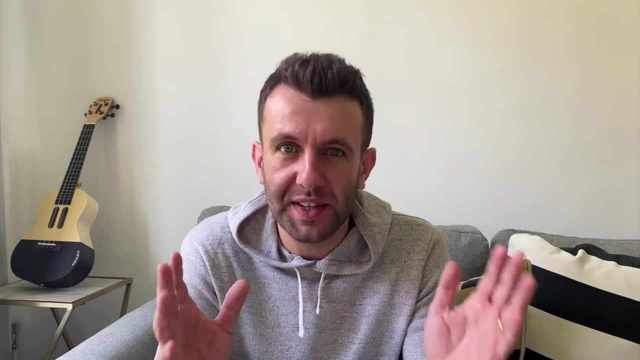 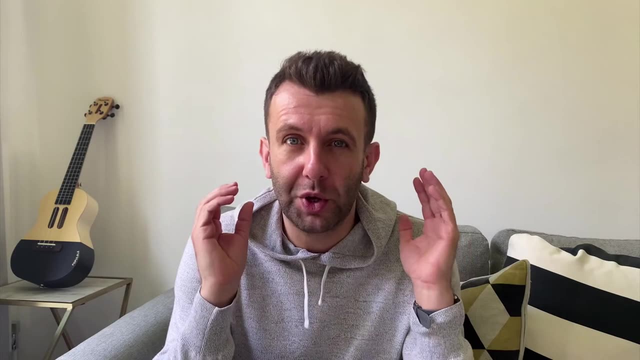 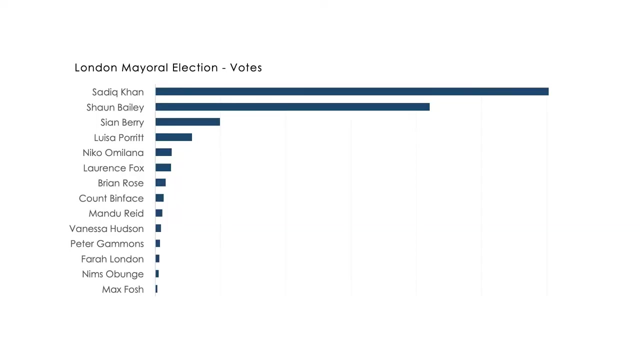 However, if you absolutely must have between seven and fifteen different data points, flip your vertical bar chart on its side and you have a horizontal bar chart. Really, though, the best when you want to communicate ranking. so things like election results, like this chart about the London mayoral elections that shows the candidates ranked by votes, They're also great for. 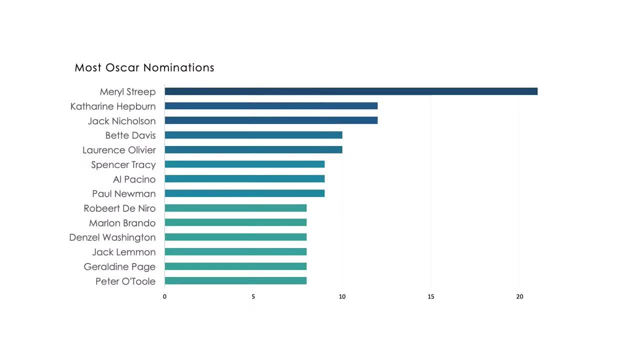 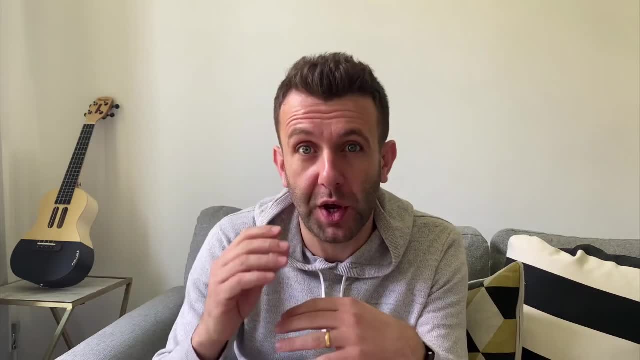 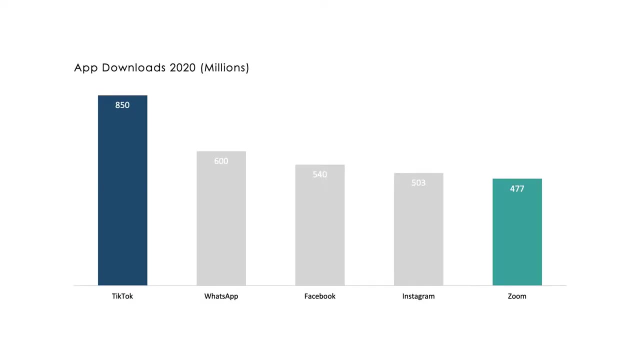 showing things like performance stats, like sales performance, or this example here which shows Oscar nomination performance. You should use stacked bar charts if you want to show part to whole. so how much different elements contribute to that overall total? For example, we already showed this chart where the main message was that TikTok, not Zoom, was the most downloaded app. 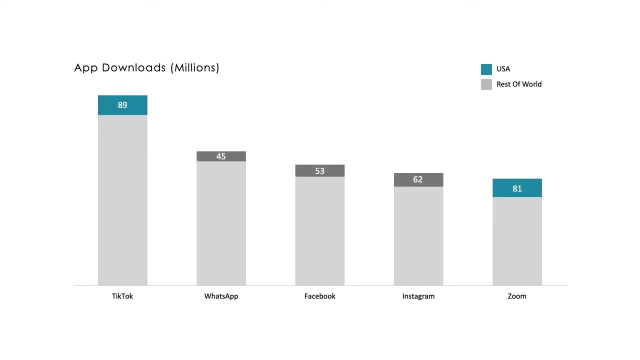 And if you were then to use a stacked bar chart and break out the downloads for the US, you still get the overall picture. but you also see that in the US the difference between the two is actually a lot smaller, which is probably why people thought that Zoom was more popular. 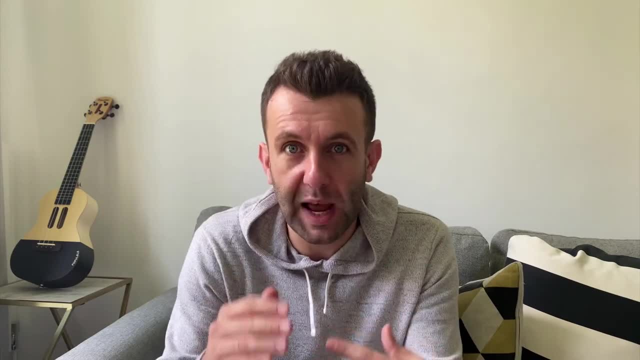 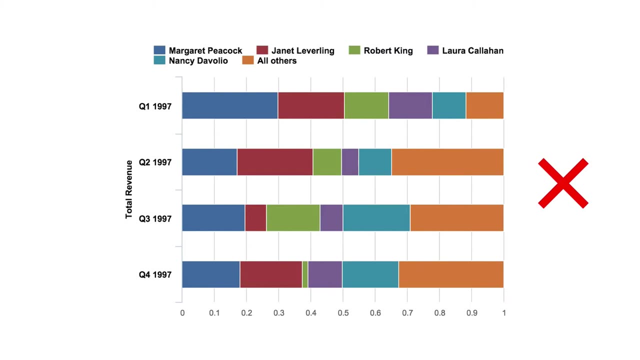 A warning though: for stacked bar charts: keep them simple. As soon as the stacked bar chart becomes far too complicated, like this one, comparing the different components becomes almost impossible and they become more or less useless. So that's bar charts. now for the second most popular chart in. 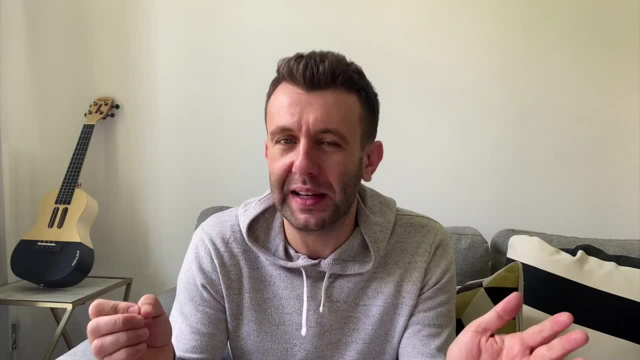 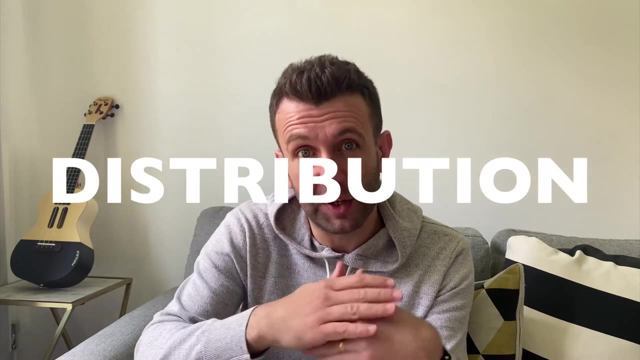 the world, which is the histogram. Now for the second most popular chart in the world, which is the histogram, Which is basically a bar chart. but if a bar chart breaks down data by different categories, histograms should show the distribution over a continuous variable. So things like time. 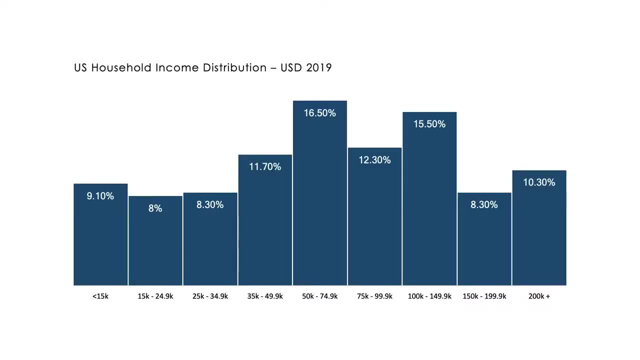 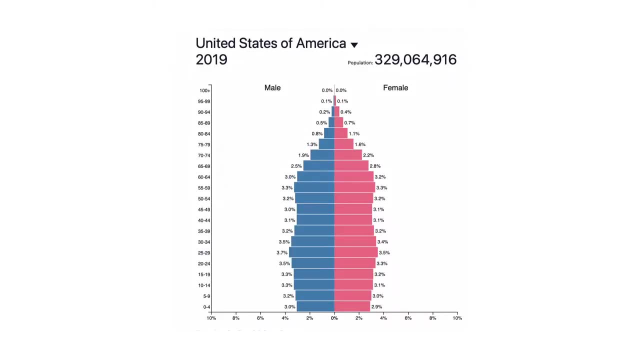 age weight. These charts are great to understand things like this one showing the income distribution in the US and, probably most famously, population distribution. Like this one showing data for the US where age is on the y-axis and population on the x-axis. It's split by. 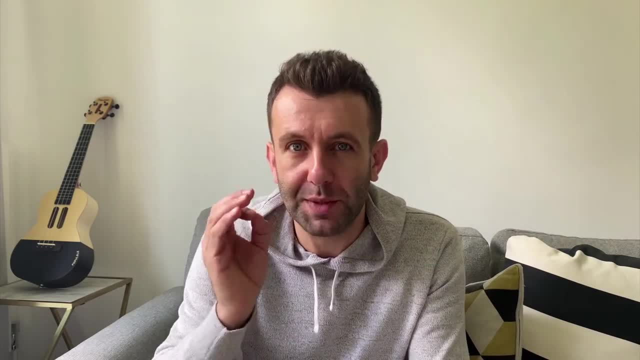 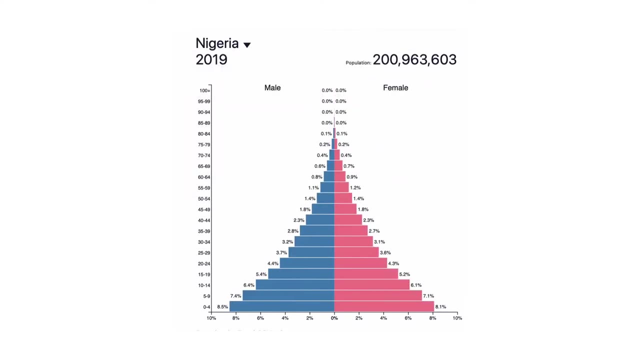 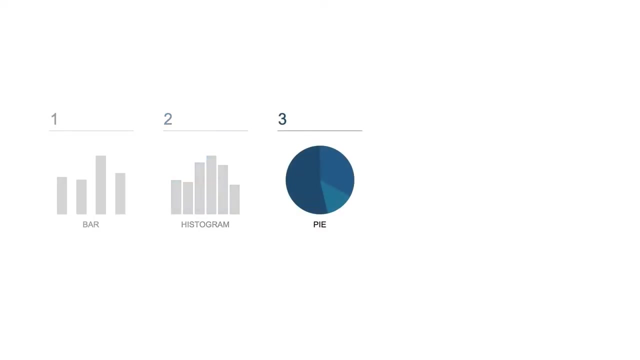 male and female, and histograms are generally less about the individual data points and more about the broader pattern that it shows. So if we quickly change this and look at data for Nigeria, you can immediately see from the pattern that Nigeria has a much younger population. I'm taking bronze. the world's third most popular chart is the pie chart. Okay, 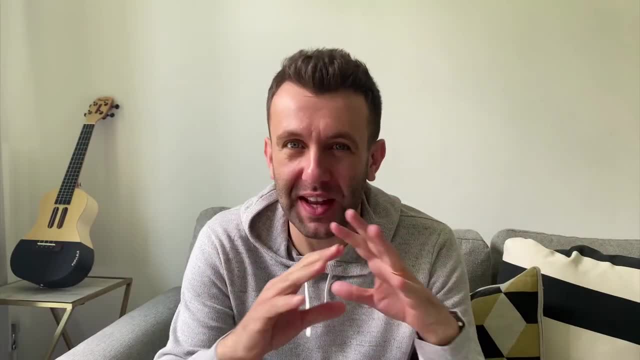 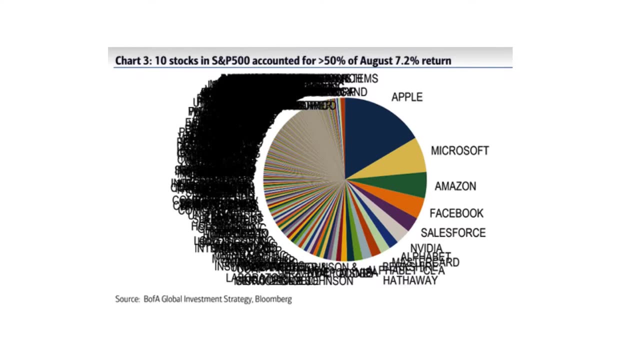 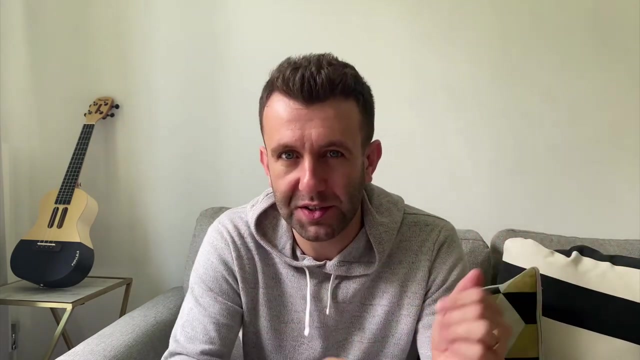 let's talk about pie charts. Pie charts are hated by data visualization experts the world over, Mainly because they're really bad at showing multiple data points like this one Fail. But also our brains aren't really very good at comparing things like areas and angles, And here's a challenge for you. So look at this chart here and quickly work out. 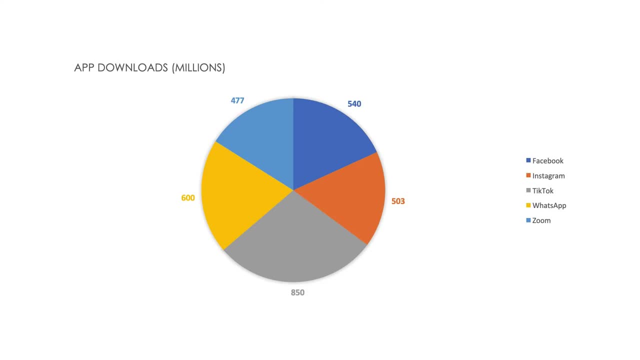 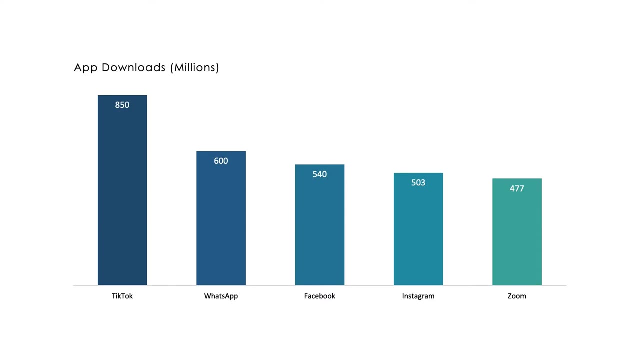 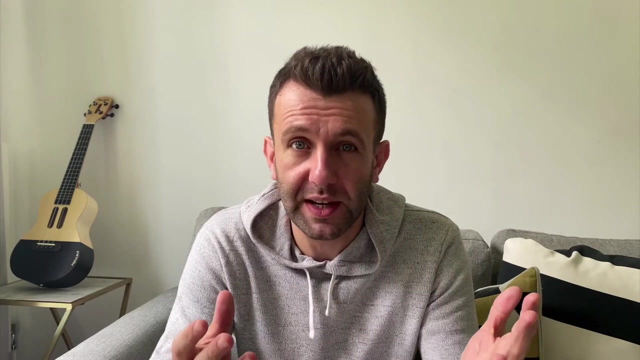 which was the third most downloaded app Three, two, one times up. Okay, now look at this one, which is showing exactly the same data, and tell me now which is the third most downloaded app. Three, two, one. Bar charts are just much better than pie charts for communicating data, But if you 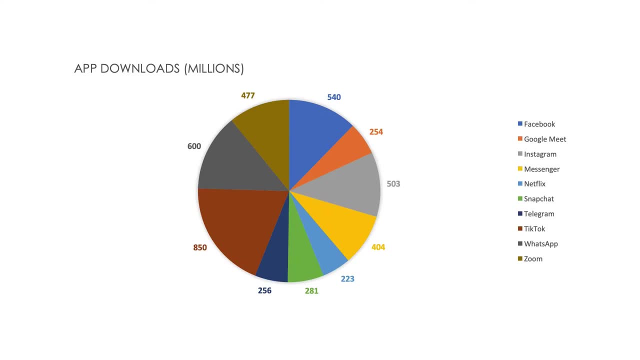 absolutely must use one. follow these tips: Firstly, never use more than five data points. Then rank the values in order where the biggest segment begins, in the top right hand corner. Then make sure you put all labels next to the segments, which means you can also remove the key And then use. 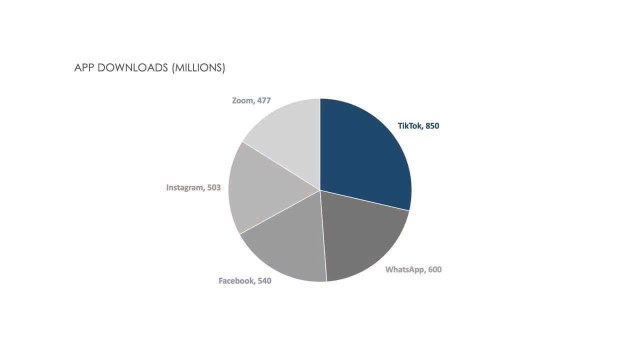 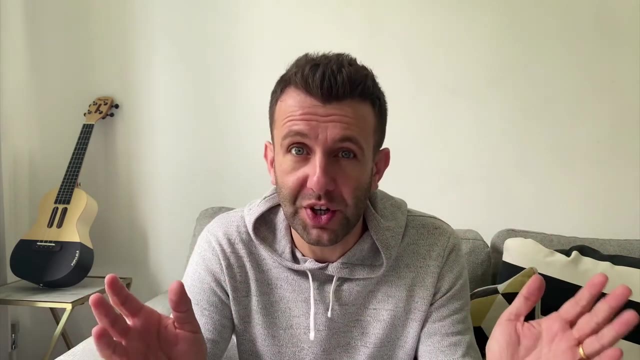 colors to help you communicate what you want to point out. In fourth place, we have scatter plots. Now, if you're looking to show correlation or how two things relate to each other, then scatter plots are your best mate. They can be used to either show that there is 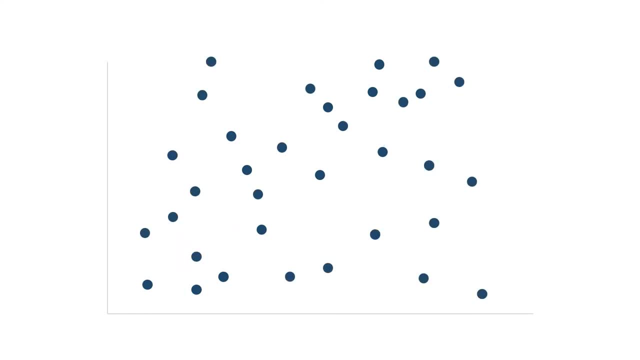 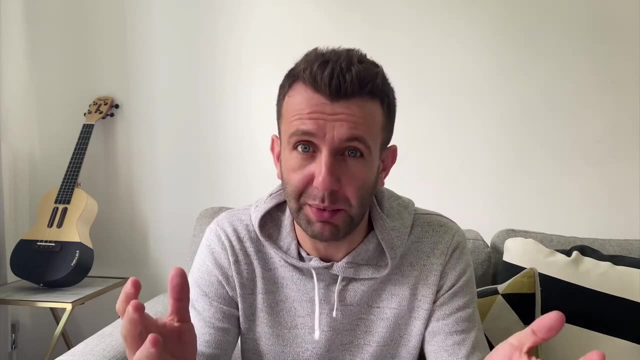 a correlation or that there isn't a correlation, To show clustering trends Or to spot outliers. They're probably one of the most persuasive charts to use if you want to convince somebody of something. The world's fifth most popular chart is the line chart, So if you 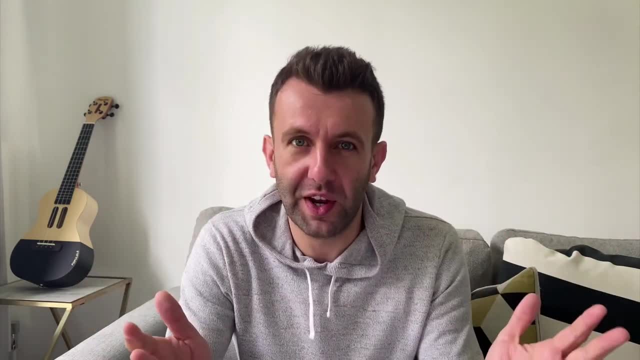 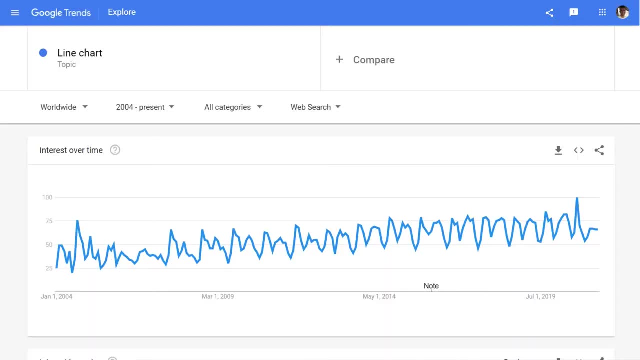 want to show how something changes over time, then go for the line chart. It's great for showing things like stock market price visitors to your website. or, if you want to go really meta. This is a line chart showing the search volumes of the term line chart since 2004.. So we can quickly see. 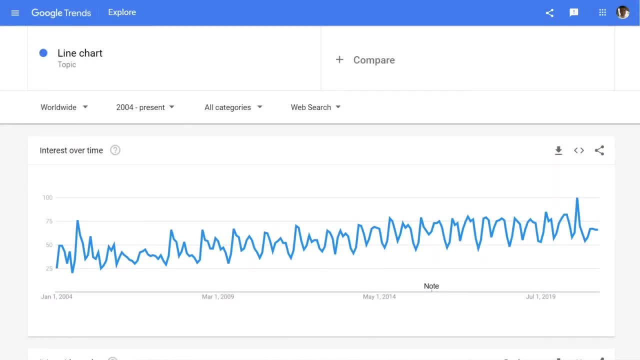 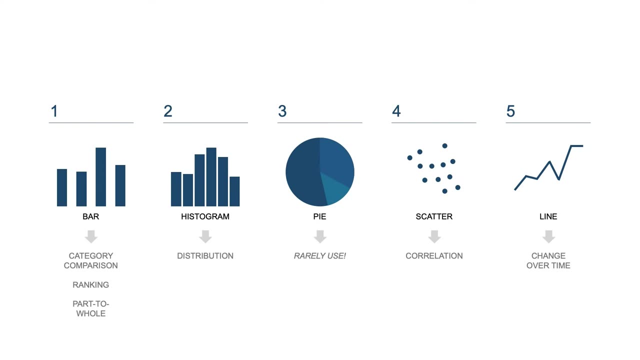 that its popularity has increased, While also being able to show how much data is being used, So dipping every December and every July. So these are the world's five most popular charts. It's not to say there aren't other charts that you can use, But unless you're a data viz master. 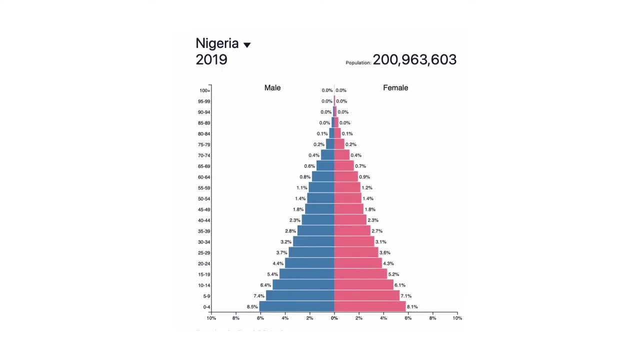 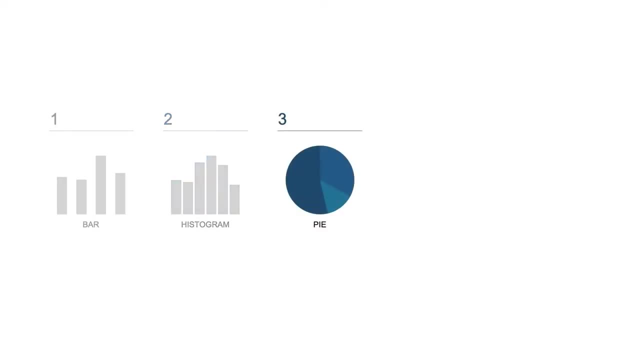 So if we quickly change this and look at data for Nigeria, you can immediately see from the pattern that Nigeria has a much younger population. I'm taking bronze. The world's third most popular chart is the pie chart. Okay, let's talk about pie charts. 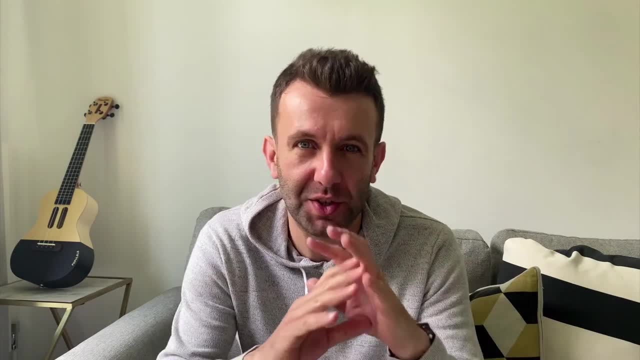 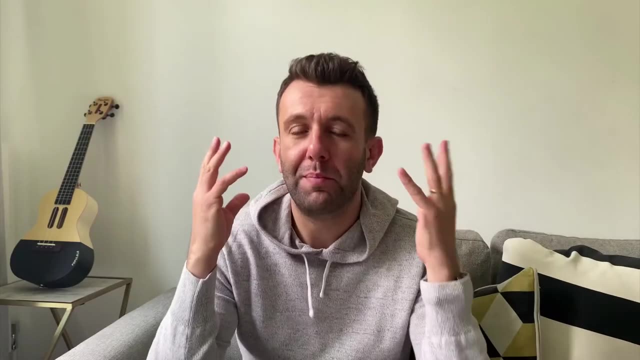 Pie charts are hated by data visualization experts the world over, mainly because they're really bad at showing multiple data. points like this one Fail. But also our brains aren't really very good at comparing things- Things like areas and angles- And here's a challenge for you. 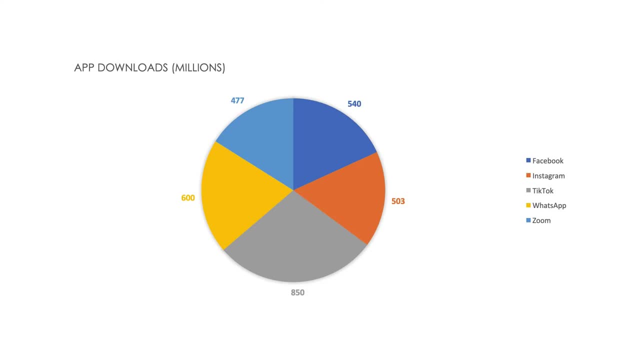 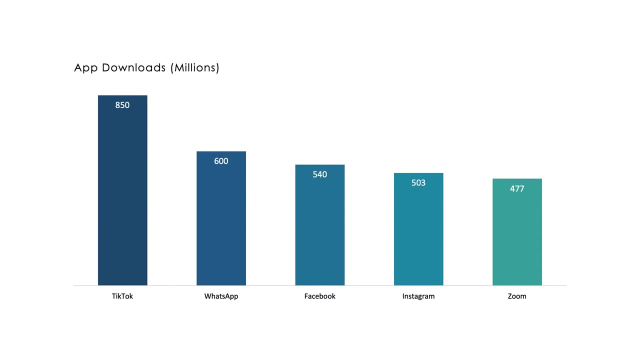 So look at this chart here and quickly work out which was the third most downloaded app. Three, two, one times up. Okay, now look at this one, which is showing exactly the same data, and tell me now which is the third most downloaded app. 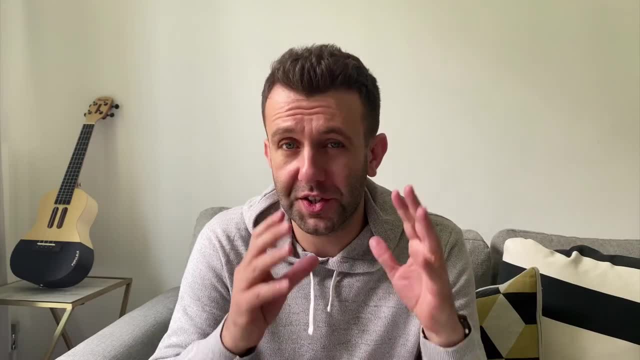 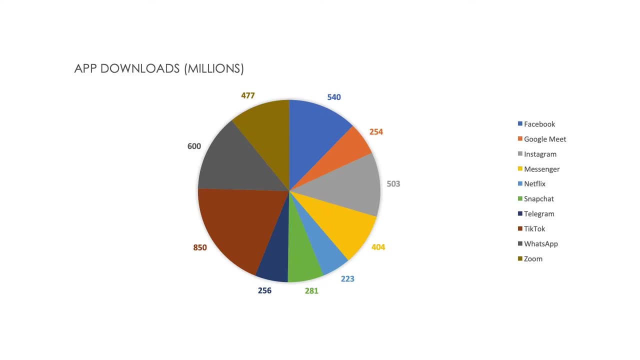 Three, two, one. Bar charts are just much better than pie charts for communicating data, But if you absolutely must use one, follow these tips. Firstly, never use more than five data points. Then rank the values in order where the biggest segment begins. 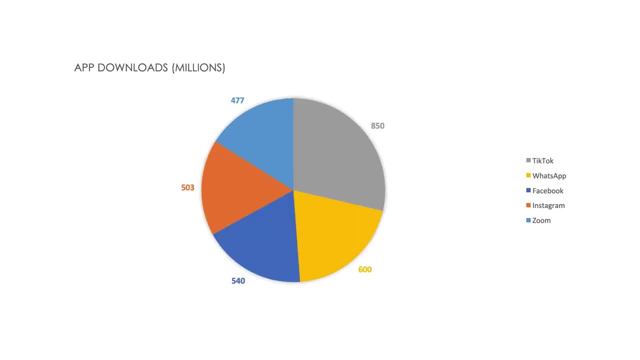 in the top right-hand corner. Then make sure you put all labels next to the segments, which means you can also remove the key And then use colors to help you communicate what you want to point out. In fourth place, we have scatter plots. 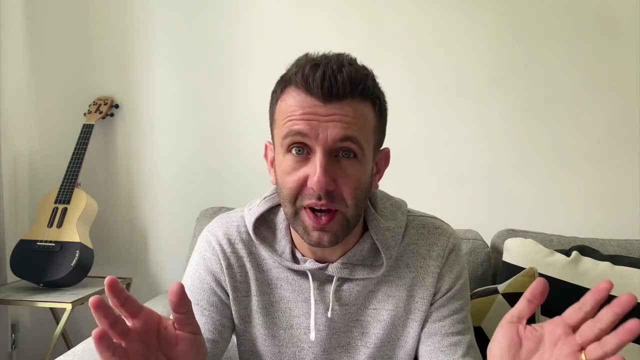 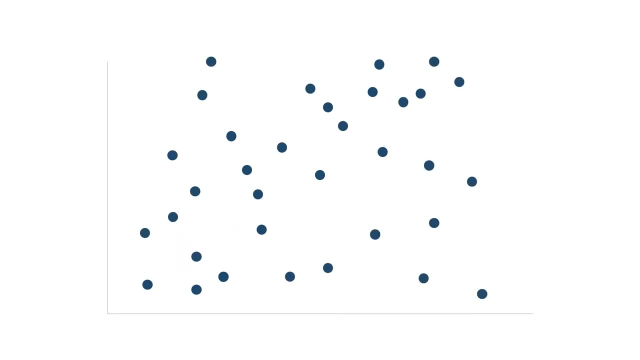 Now, if you're looking to show correlation or how two things relate to each other, then scatter plots are your best mate. They can be used to either show that there is a correlation or that there isn't a correlation, to show clustering, clustering trends, or to spot outliers. 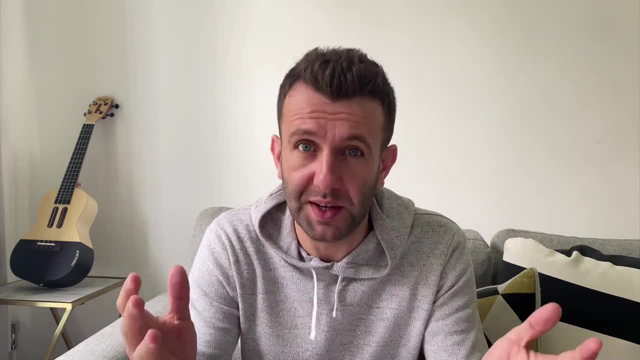 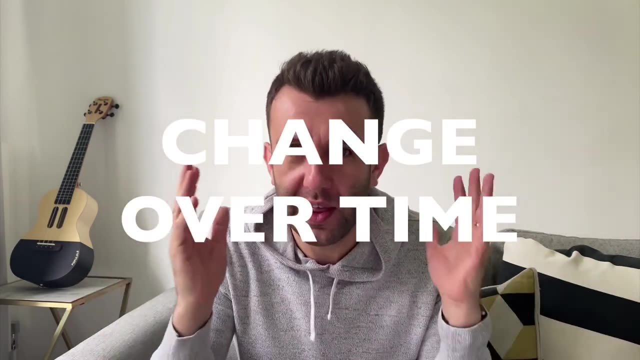 They're probably one of the most persuasive charts to use if you want to convince somebody of something. The world's fifth most popular chart is the line chart. So if you want to show how something changes over time, then go for the line chart. 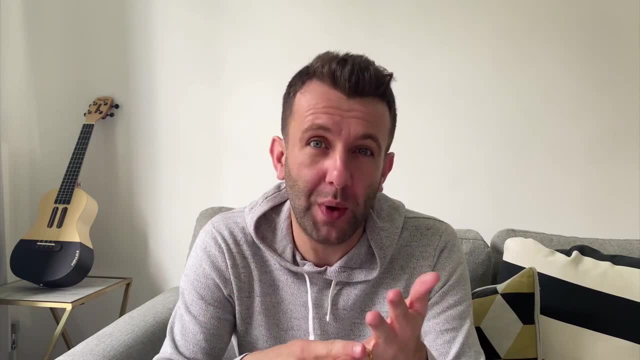 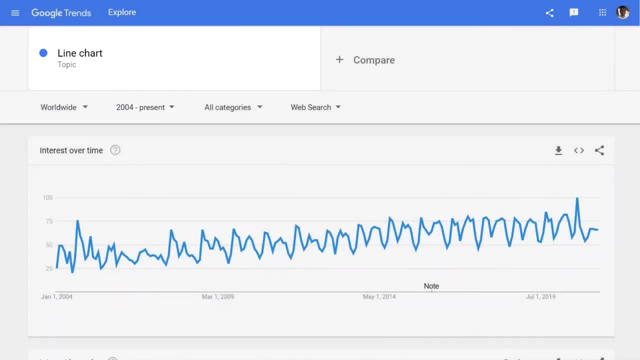 It's great for showing things like stock market price visitors to your website. or, if you want to go really meta, This is a line chart showing the search volumes of the term line chart since 2004.. So we can quickly see that its popularity has increased. 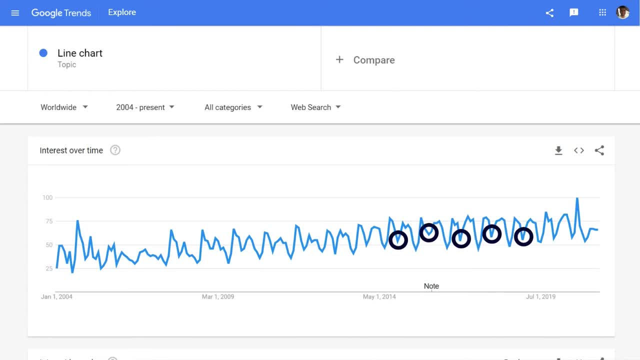 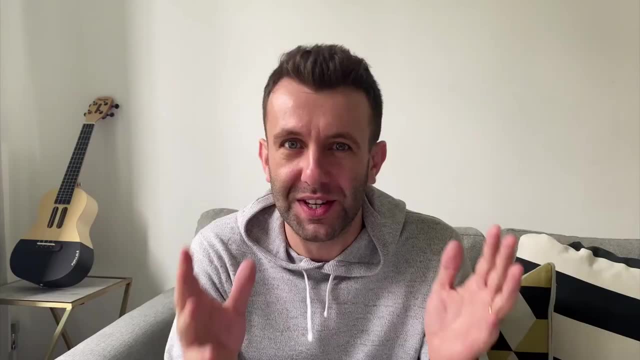 While also dipping every December and every July. So these are the world's five most popular charts. It's not to say there aren't other charts that you can use, but unless you're a data viz master, stick with these and spend that extra time.